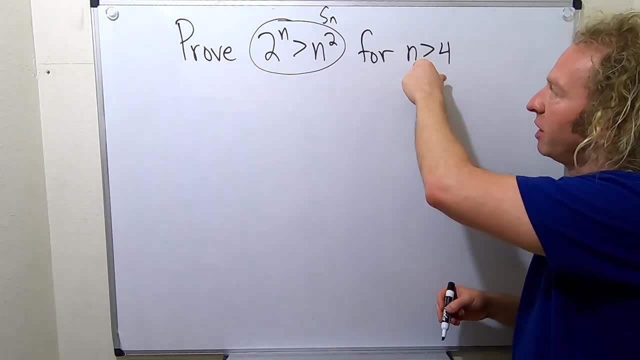 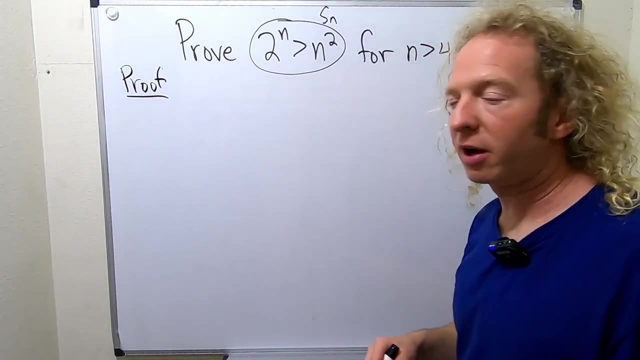 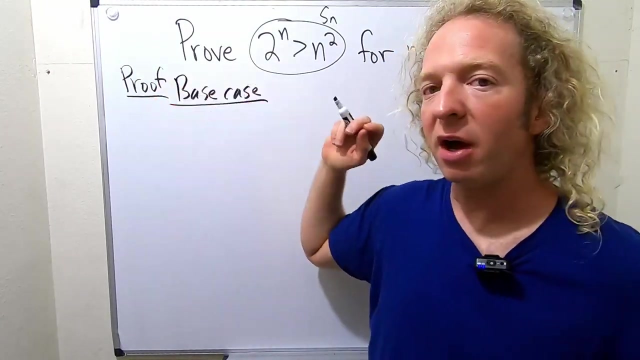 And induction shows that a statement is true for all n, In this case all n bigger than 4.. All right, let's do the proof, So proof. So I like to start my induction proofs by writing down the base case, So base case. The base case is the starting point, right, You show it's true for the smallest integer that you're working with. 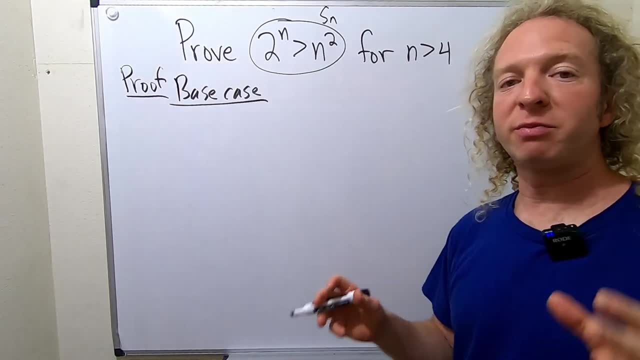 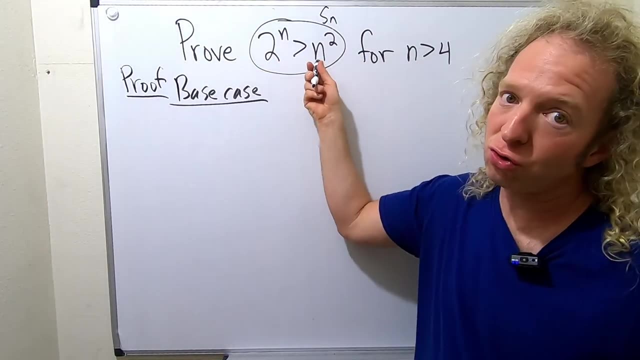 So in this case, the smallest integer we're working with is 5, right, The smallest positive number bigger than 4 is 5.. So you have to show that s sub 5 is true. So you just have to show that this is true when n is equal to 5.. 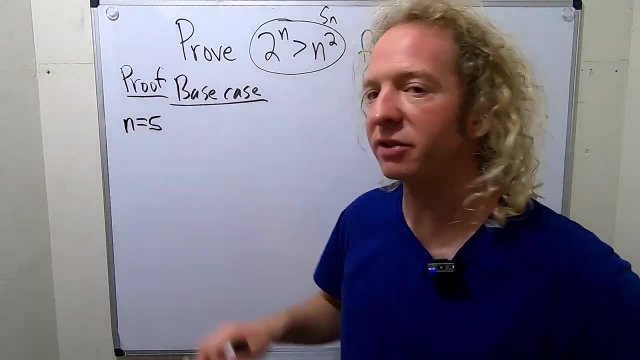 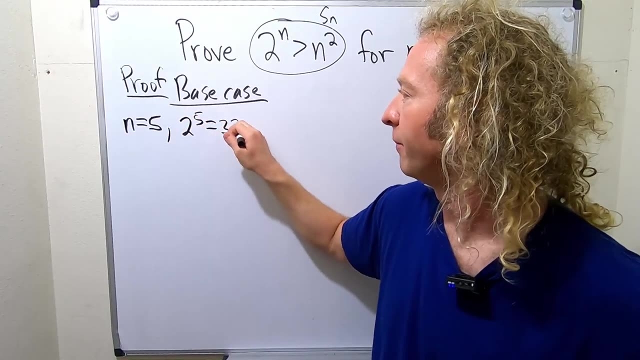 Okay, So when n is 5,, let's write it down like that: n is 5, we have 2 to the 5, right? So what is that? Let's see. So 2 to the 5 is 32, right? Okay, no big deal. 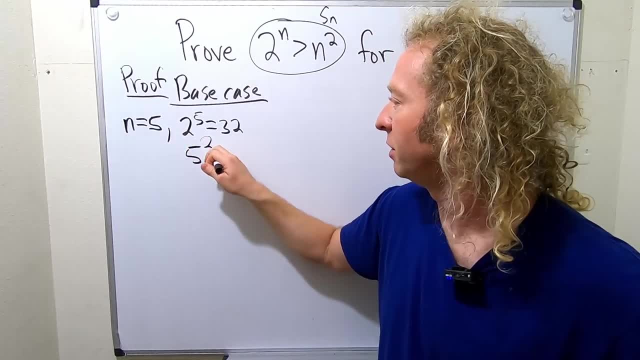 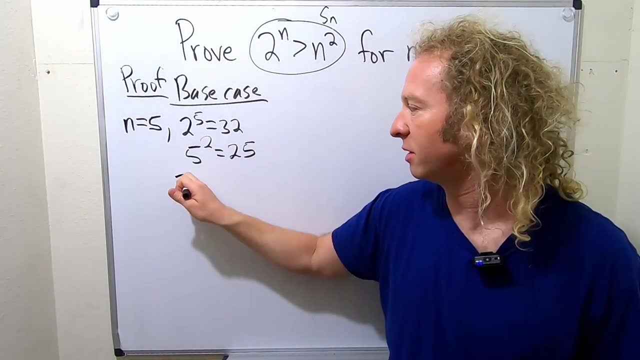 What about this right? Well, this bad boy is going to be 25, right? Ah, beautiful stuff. right, It worked. This is bigger than this right, So I'll say it. It seems kind of silly, but who cares? 32 is bigger than 25.. Boom. 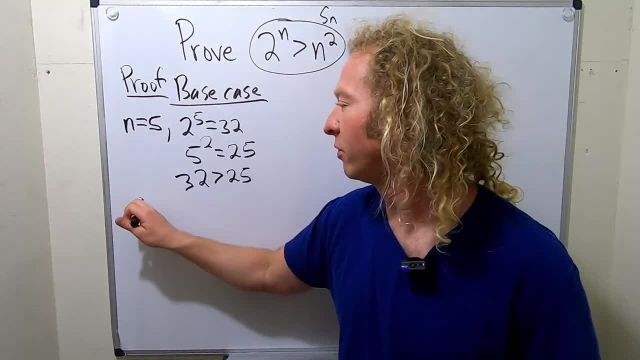 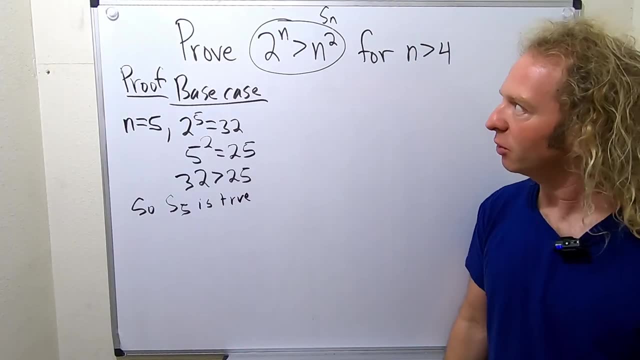 So that means that the statement is true when n is equal to 5.. So I'll even write it this time. So s sub 5 is true. Boom, The base case is proven. The base case is pretty easy. Most people can do the base case. 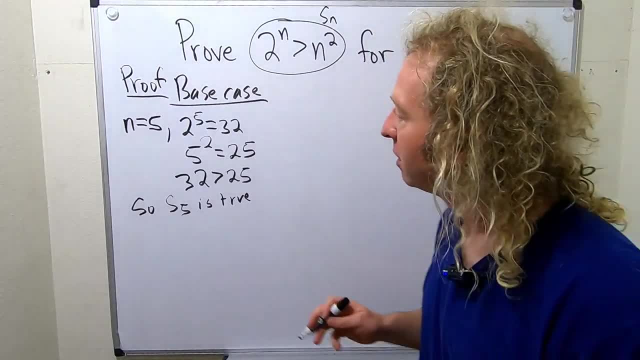 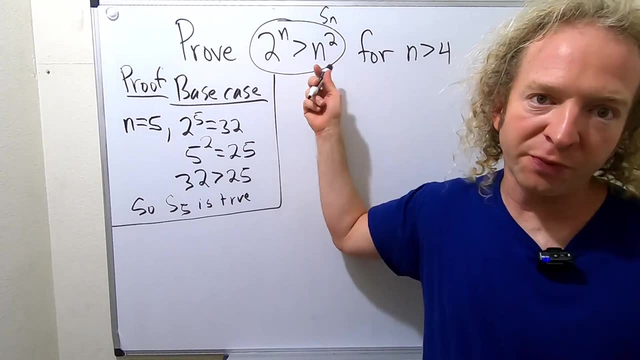 The hard part is the inequality part. All right, So now we have to do the induction hypothesis. That's pretty easy also. So the induction hypothesis is: basically: we assume that this statement is true for some positive integer greater than 4.. So I'm going to write: induction hypothesis. 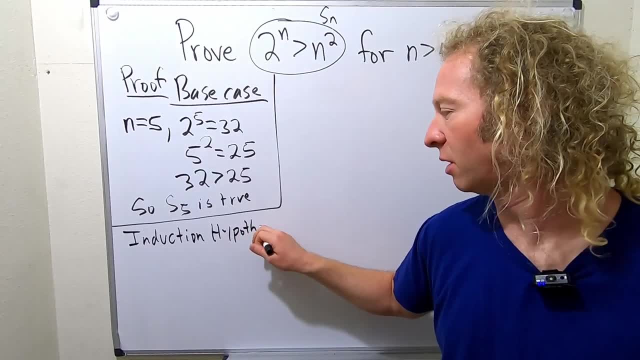 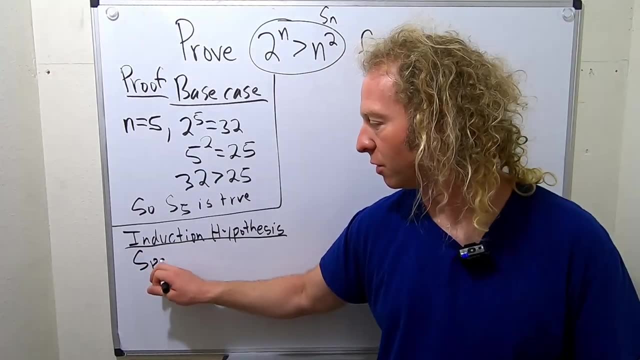 So induction hypothesis, I'll spell it Completely: Hypothesis It's not, Let's be pro, Let's do it right. So suppose, so suppose, suppose that this is bigger than this right. So 2 to the k is bigger than k squared. 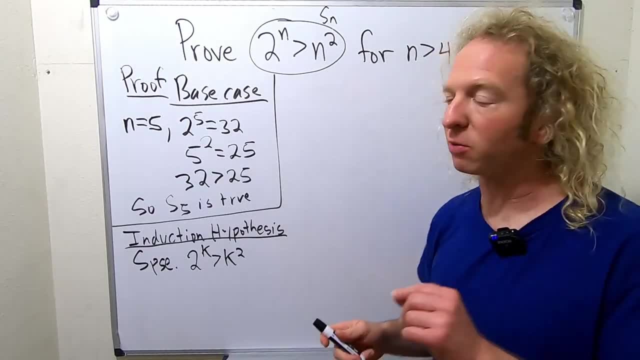 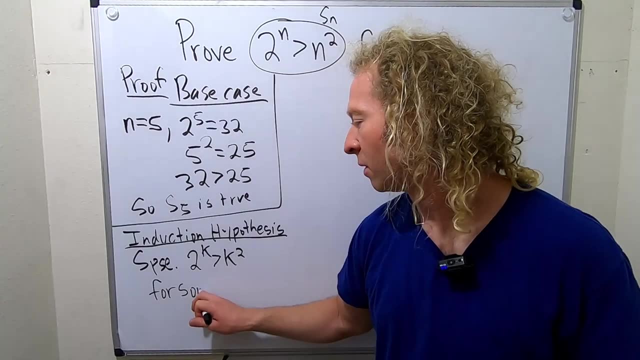 And it's for some k bigger than 4.. And in this particular problem, these inequality problems, you're actually going to use that very, very heavily. So for some k bigger than 4.. So we're actually going to need this. 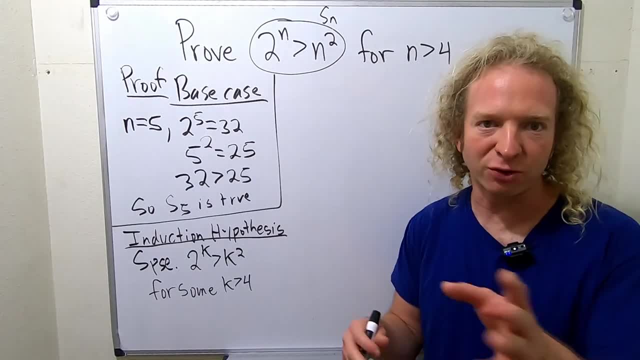 I know a lot of times induction proofs Learning, it's, like you know, for k equals 1 is the base case And, like you never use it again, really right, It matters. It's a big deal in this problem. 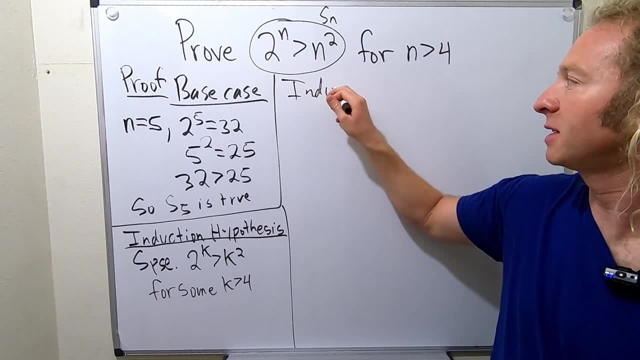 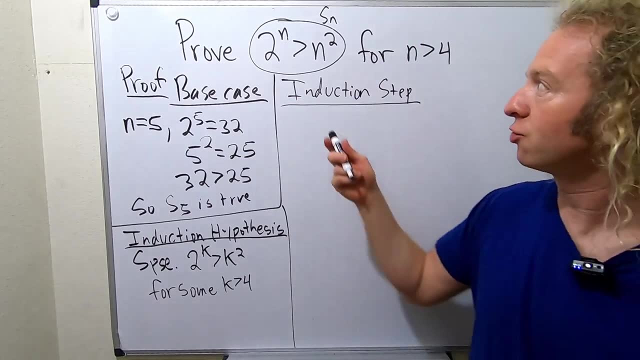 All right, The induction step. The induction step. I like to break it up into three steps just for clarity. So the induction step: This is where we have to show that our statement is true when n equals k plus 1.. Okay, 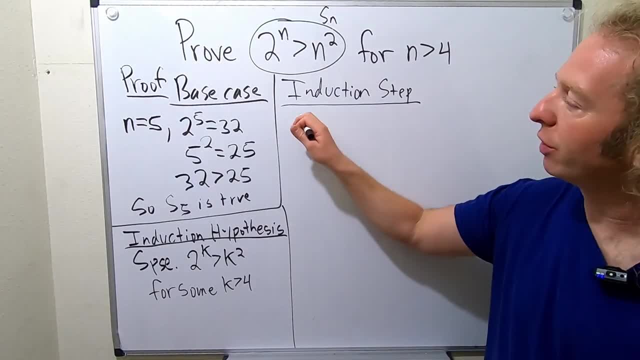 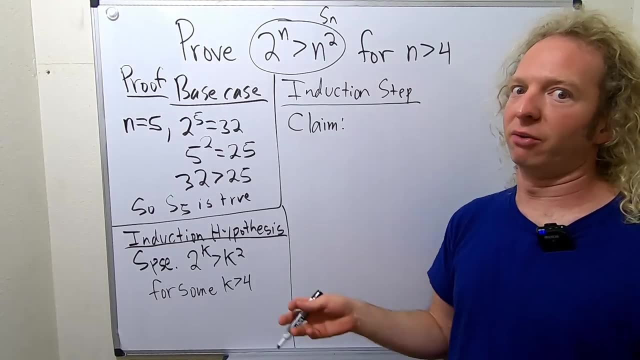 So I'm going to write down what we have to show. So it's really important to write claim before you do that, So that the reader knows that you're not just like, oh you know, so they know that you know what you're doing, right. 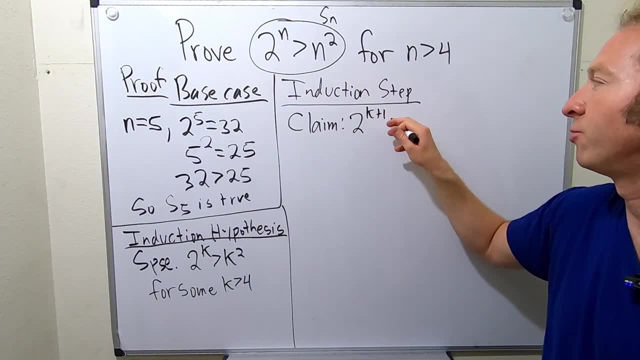 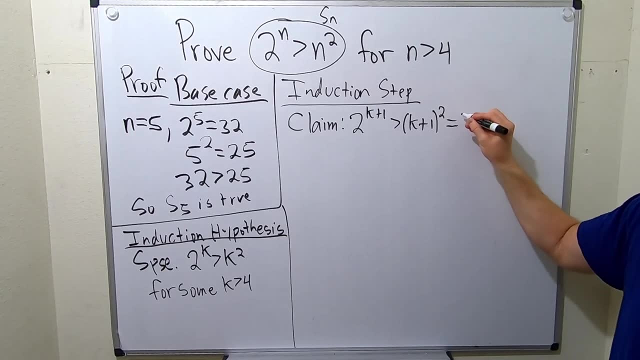 So claim, because this is what we have to prove. We technically can't write this down unless it's been proven, So we have to prove this, Just for our own benefit. we should multiply this out. It's pretty easy, right. 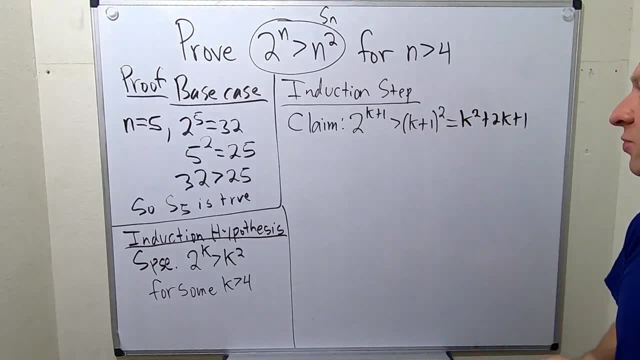 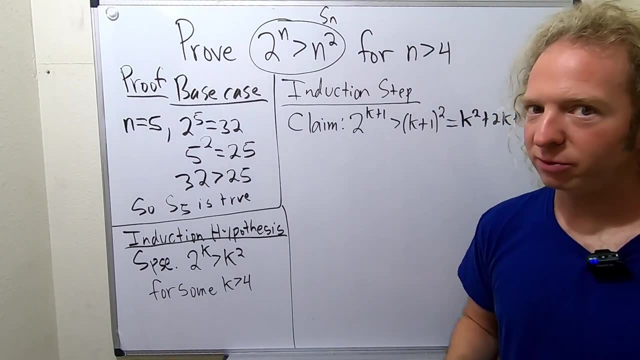 You square the first one, you multiply these and double them, and then you square the last one. Okay, So that's what we have to prove, All right? So How do we do that? I don't know. Let's just try. 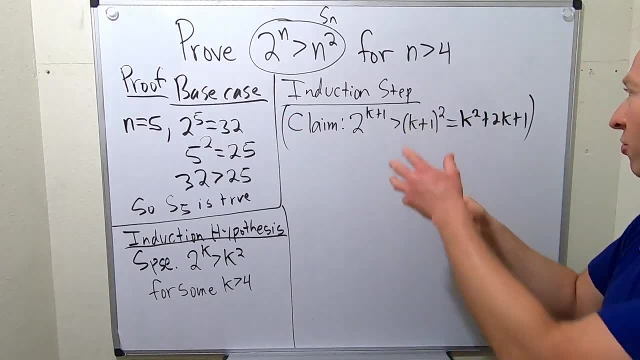 So now we're just going to try. So I'm going to start with this and I'm going to try to show that it's bigger than this. We somehow have to use this and this, So it's just a matter of working through it. 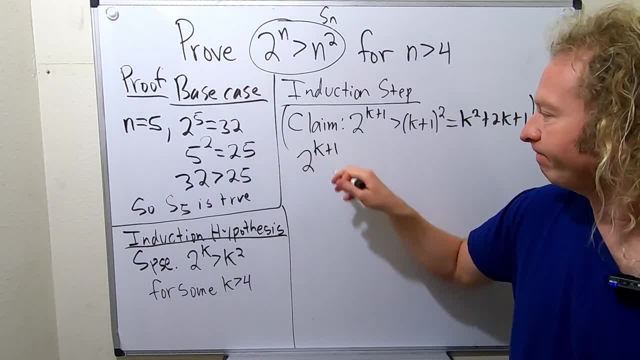 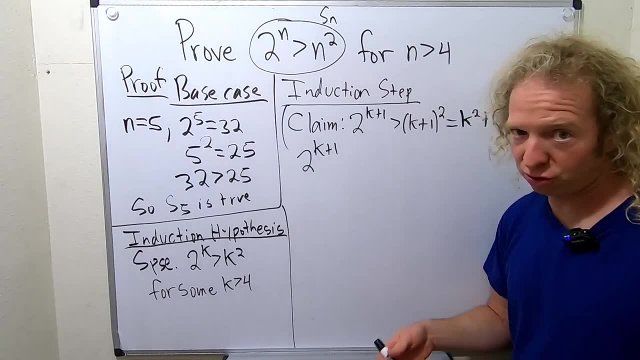 Let's do it. So we have 2 to the k plus 1.. Okay, So what do we do next? Well, we know we have to use this right, So the natural thing to try- right to try- is to write this, as you can write it like this: 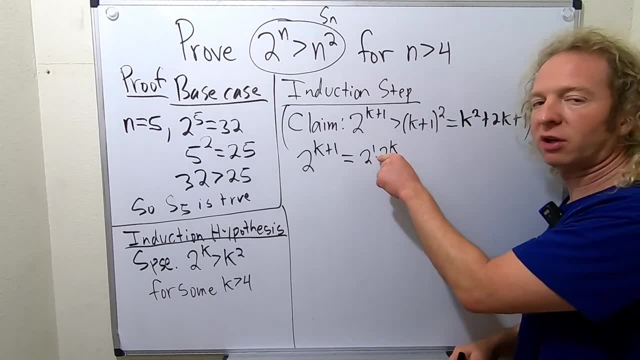 2 to the 1 times 2 to the k, right? It's a clever algebra trick, right? Because when you multiply these you add the exponents. right, It's 1 plus k or k plus 1.. 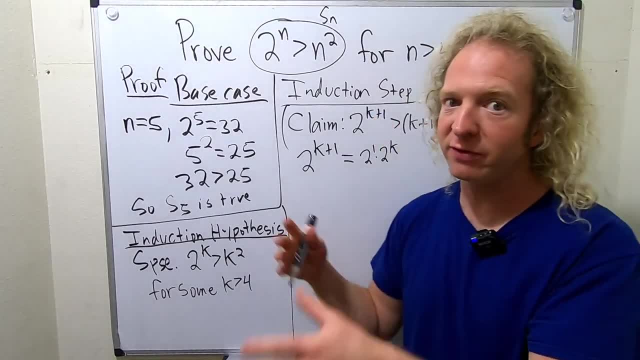 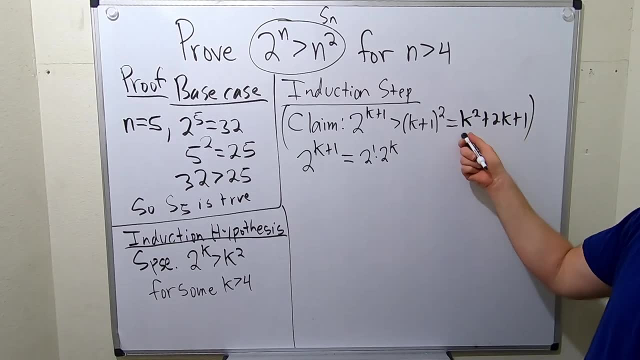 So that's usually no matter what you're doing. if you're doing inequality proof, even similar to this one, right, It's a good first step. So now, what do you do? You say, okay, you're trying to show it's bigger than this, right. 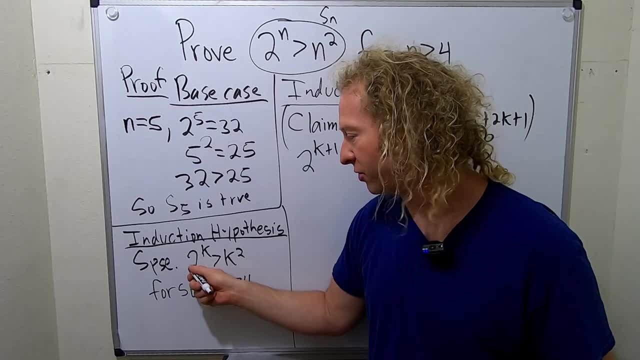 And you have 2 to the k here. You have 2 of them, though, right, You have 2, 2 to the k here, Okay, So here you have 1 of them. So what you can do is you can separate this. 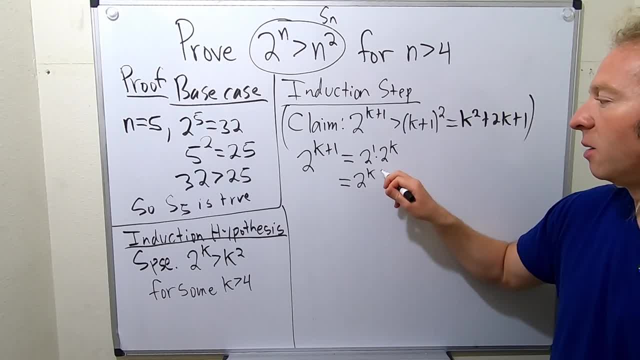 This is, there's 2 of these, So it's really 2 to the k plus 2 to the k, And I'd say, why'd you do that? Because we have 1 of them here, right Here we have 2.. 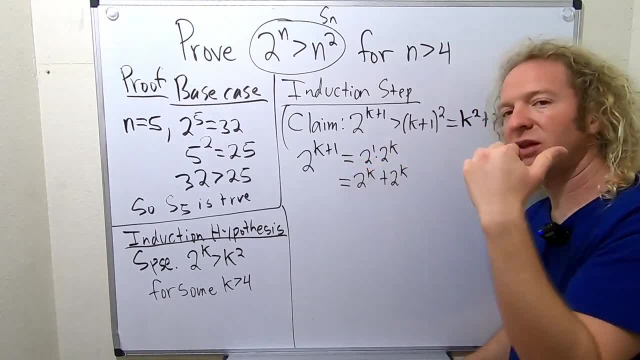 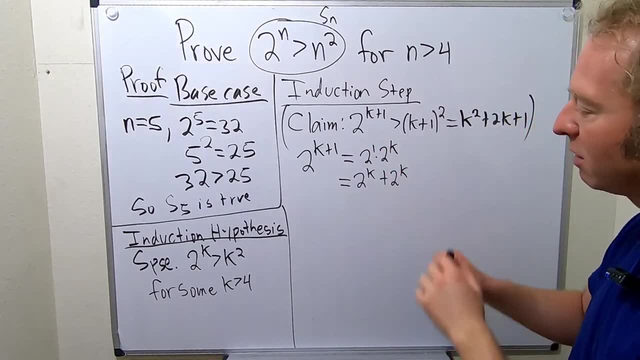 So now we have 2 to the k plus 2 to the k is 2 times 2 to the k. Think of it like x, right? x plus x is 2x. x plus x is 2x. People have a hard time with this stuff. 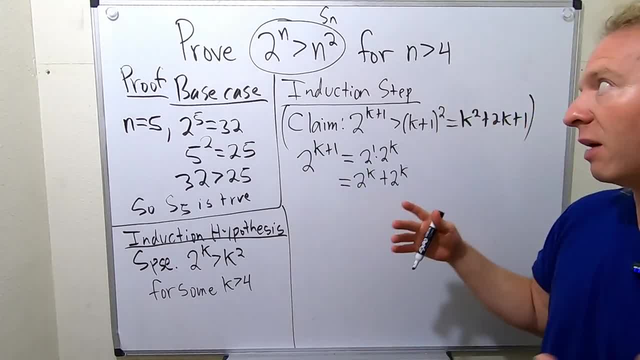 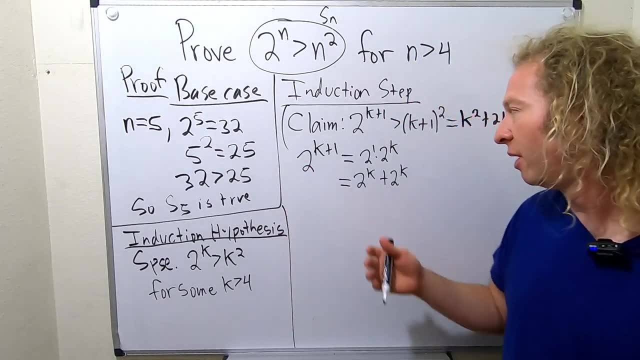 In general, these inequality proofs are extremely difficult. When I was first learning this stuff thousands of years ago, I didn't get it. I stayed up all night, I tried, I tried. I could never understand it right, So hopefully it makes sense. 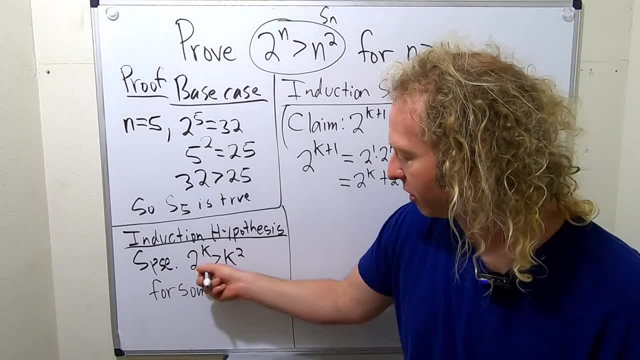 So x plus x is 2x. Okay, 2 to the k is bigger than k squared, So you can put a greater than here. This is the part I used to have a hard time with, And you can just replace it. 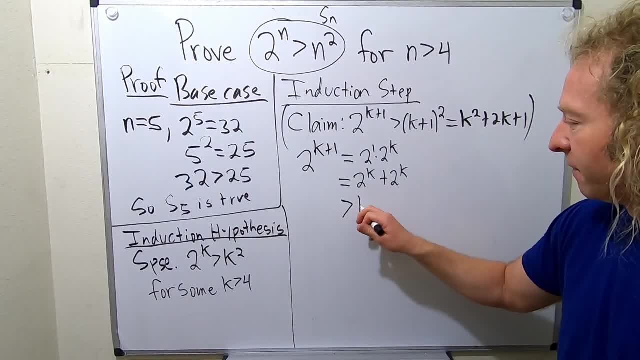 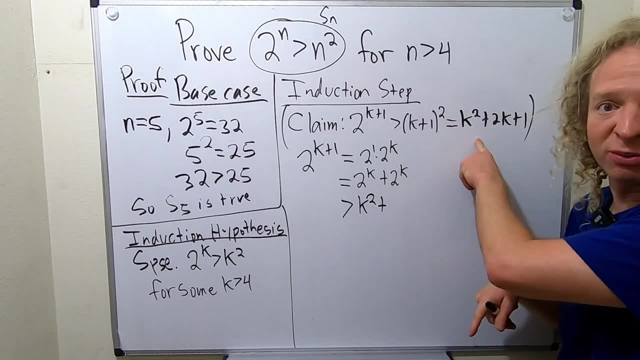 You're allowed to do that in math. okay, I used to not understand that And we can do the same thing here. Let's go ahead and replace this one. I'm thinking we're not going to need any 2 to the k's anymore, right? 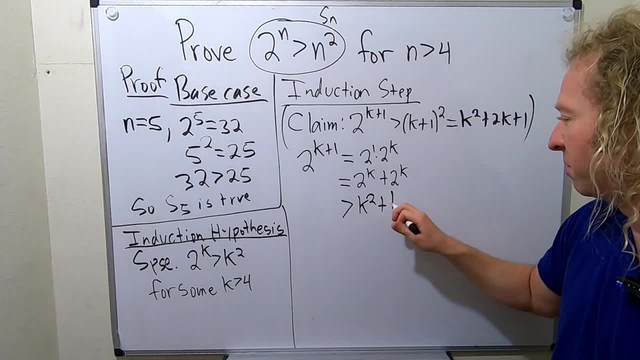 Because there's none here. That's where we're going, So let's go ahead and replace both. I was only going to replace one, but I thought: wait, what am I doing, right? Like we don't need these anymore, so we can replace them. 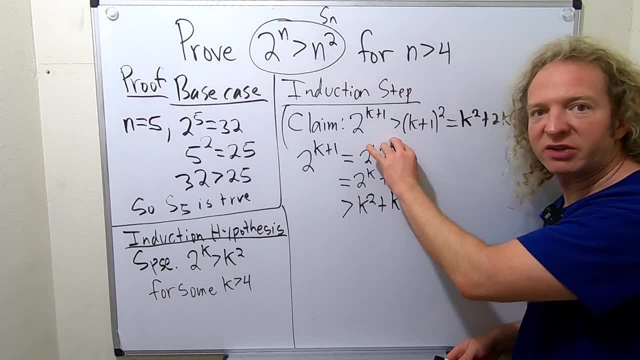 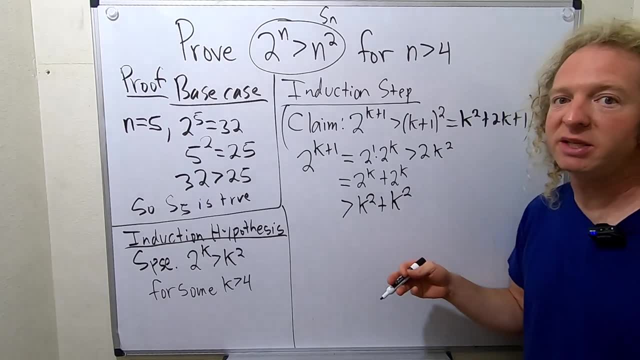 Actually, I didn't even need to break it up like that. I could have just replaced this with k squared and we would have had 2k squared. That would have worked as well. I could have done this. That probably would have been easier. 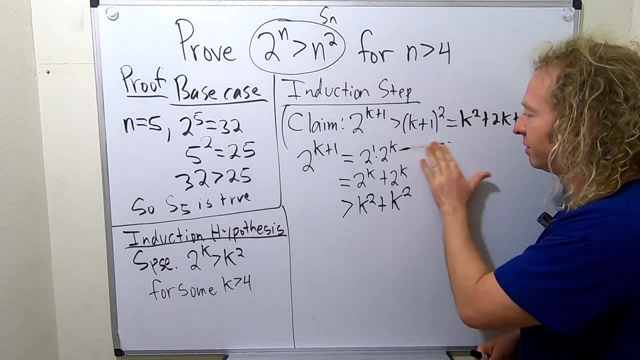 Why didn't I do it? I don't think I've done this problem before, So I think I looked at it, but I don't think I've actually worked through it. We've got that, We've got this, So that's good right. 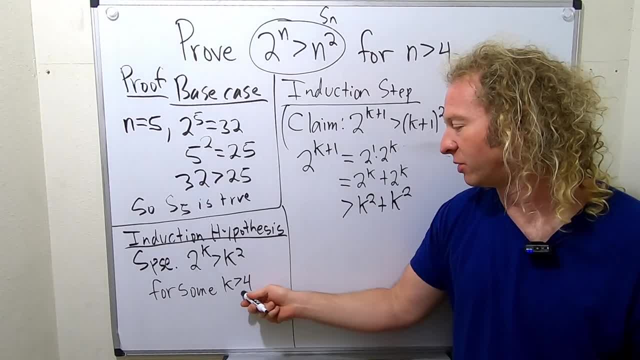 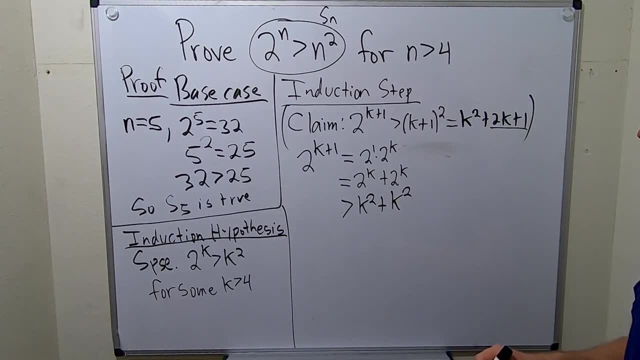 We need to get 2k plus 1.. So we somehow have to use k bigger than 4, right, We have to somehow use k bigger than 4.. So I am thinking that we can keep this k squared right. 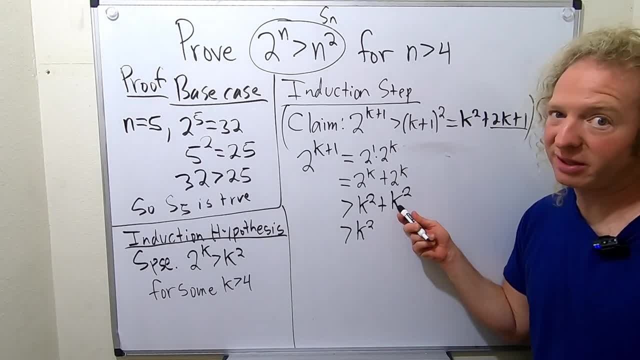 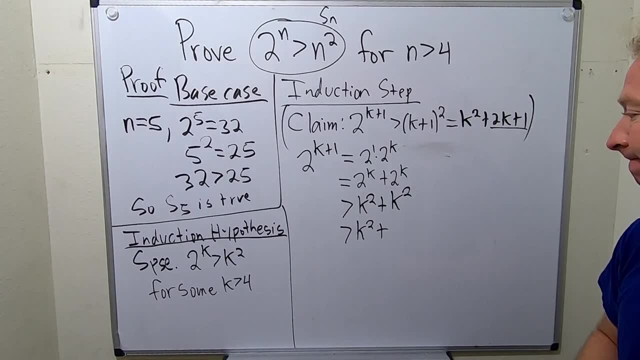 And maybe we can replace the k with 16, right, Let's see if we can do that. So this is going to be plus plus, I guess, 16. 16.. So we need to get 2k plus 1.. 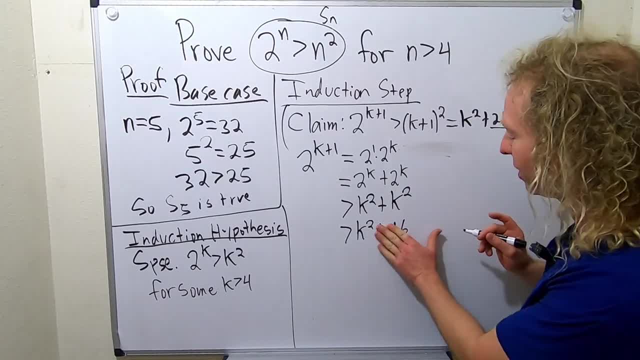 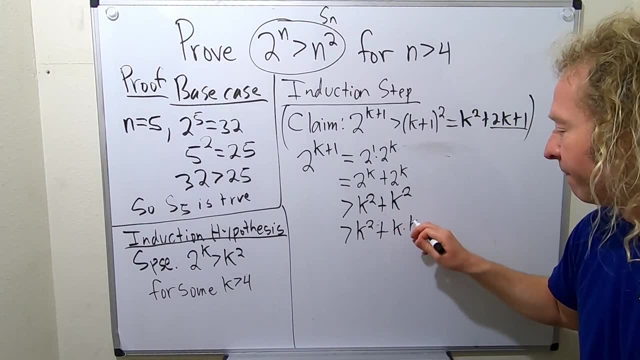 So how do we do that? Well, let's see. Actually, no, let's not do that, Let's not do that, Let's not do that, Let's. we need a k right. So let's do this right. 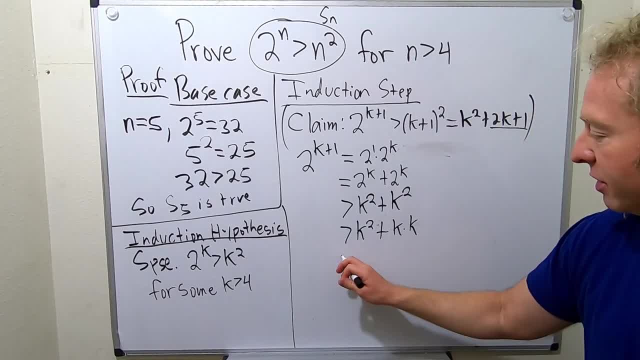 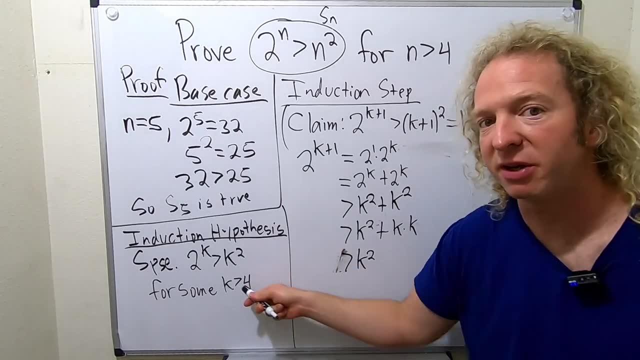 That way, we have a k right. So now this is equal to well, watch this. This is greater than replace the k with a 4, right, Because k is bigger than 4.. I almost messed up, So the reason I did that. 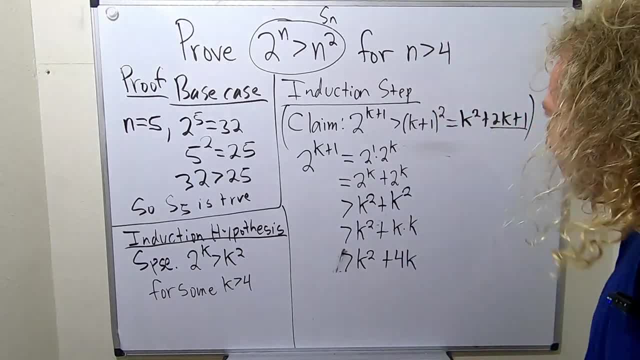 at first I put a 16 there, right. But I'm like: wait a minute, That's not going to work right Because we need a k. Like, if I put a 16 there, I place k with 4 and put a 16 here. 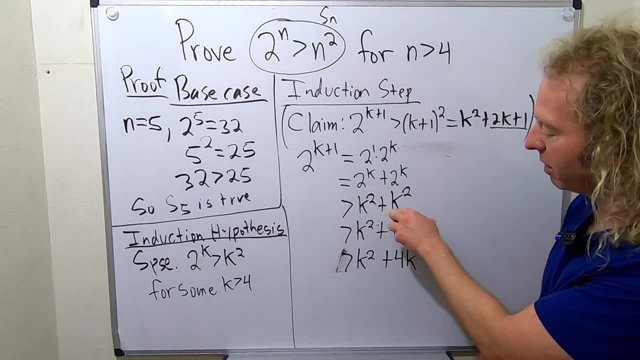 We're not going to be able to get our k back. I think, I don't know. So I think this might work better: k times, k is k squared And we can keep a k now. So how does that help? Well, 4k, we can break it up. 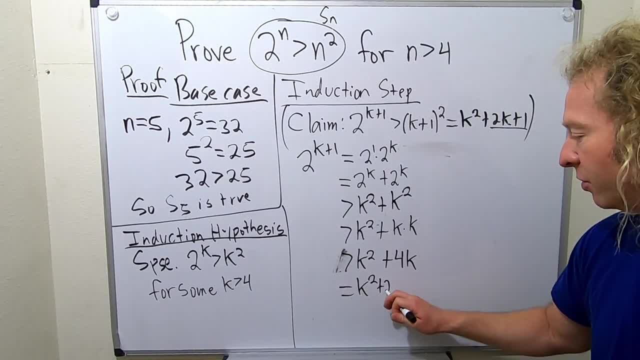 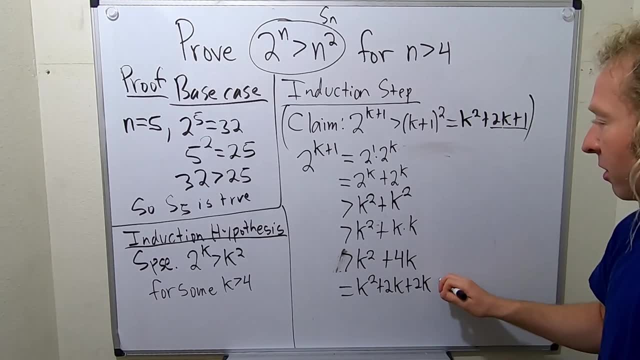 using the same technique we did before. This is k squared plus 2k plus 2k. We got it now. Look, we got k squared plus 2k, k squared plus 2k. So I'm going to come back up here. 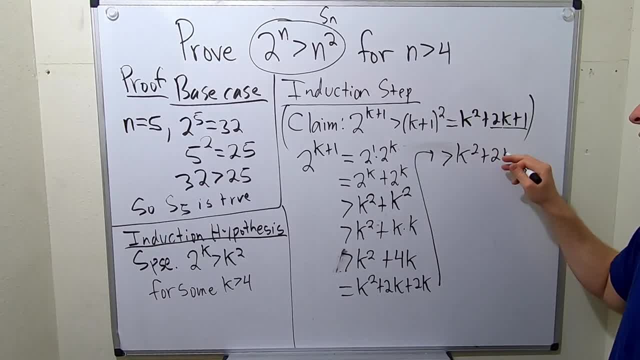 This is greater than k squared Plus 2k. Replace this k with 4, okay, So plus 8.. 2 times 4 is 8.. And now that's hard right. Is this the best way to do it? 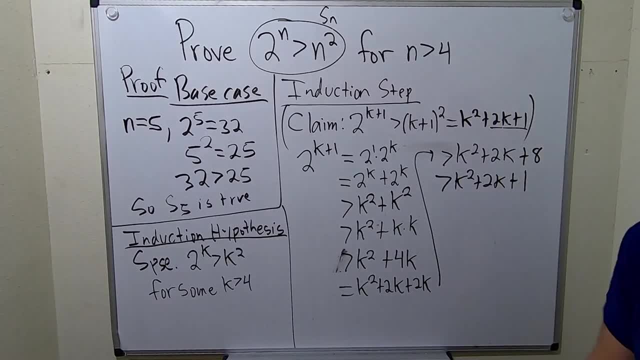 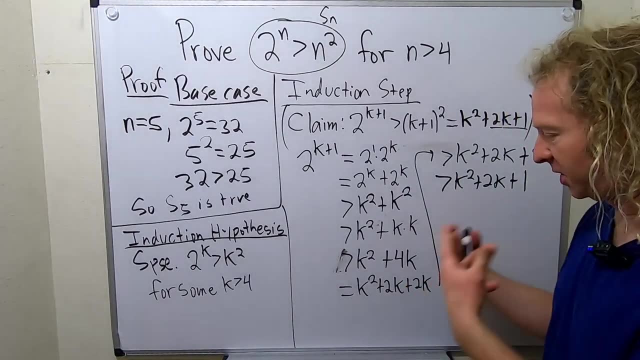 I don't know, But I know 8 is bigger than 1.. Boom, right. So brute force, right. This is just how you do it, Like, if you've never done this before, this is probably how you would do it, right. 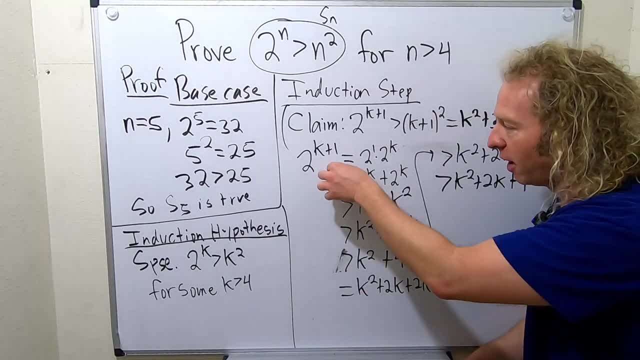 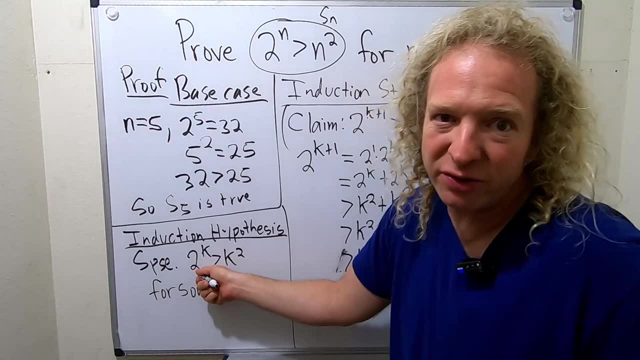 I looked at this problem and I thought I could probably figure it out. Let me make a video So you can rewrite it. first, I broke it up because I figured we only need one of these, right? I didn't need to do that, right. 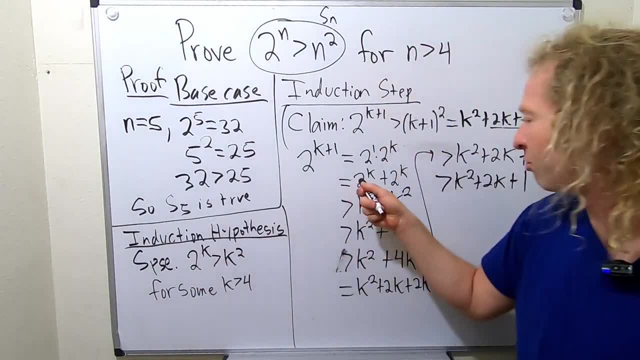 I could have just done greater than 2k squared, But I thought I only want one, So let me break it up. So I broke it up, Replaced it with k squared. I kept my k squared here. I kind of messed up here, but I fixed it right. 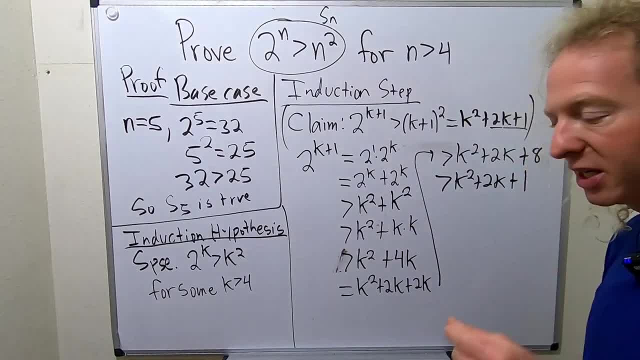 I was going to replace this with 16.. But think about it right: k squared is k times k And we need a k. So you keep a k right. Then you replace one of the k's with 4. And you say, okay, 4k. 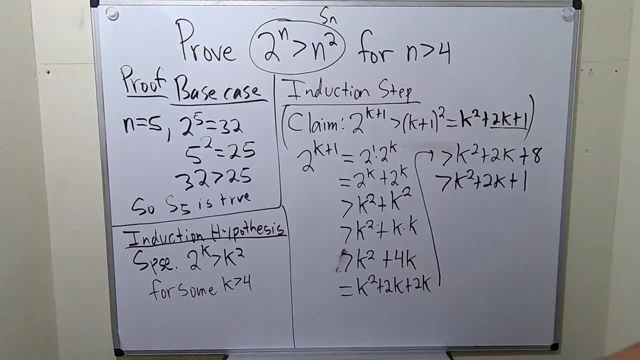 Well, you only need 2k, So 4k is 2k plus 2k right. And then you replace this k with 4.. Right, k is bigger than 4.. Gives you 8.. Replace the 8 with 1..